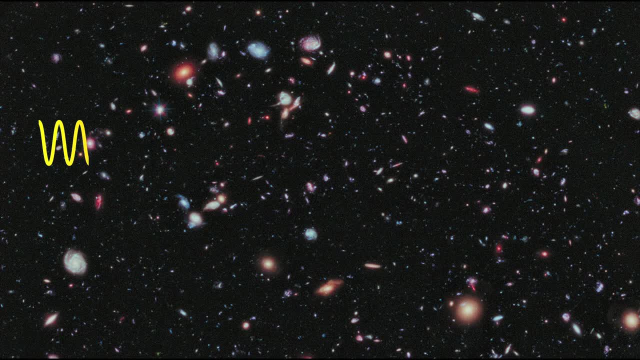 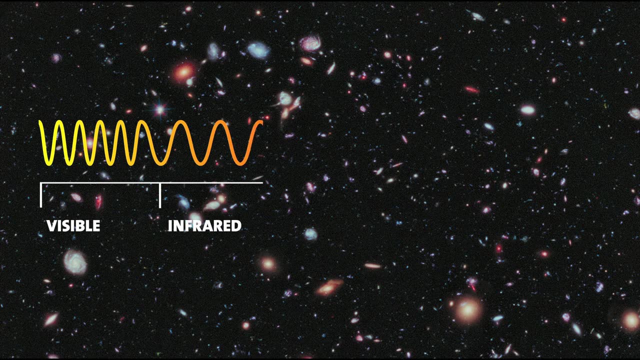 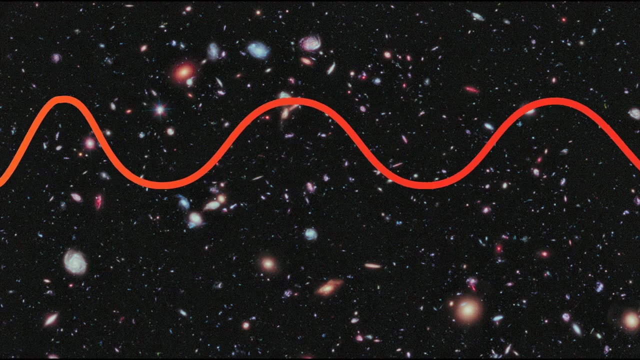 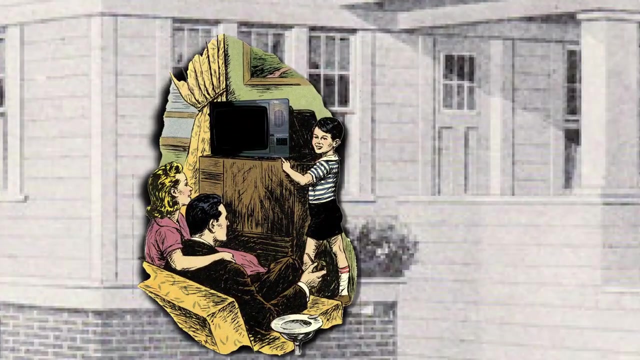 And although it was emitted, rather coincidentally, as visible light, it got stretched from visible yellow light to infrared, to microwaves, radio waves, And those radio waves pervading the universe can be detected with a microwave antenna. Heck, they can be detected with a TV antenna, an old-style on-the-air TV. 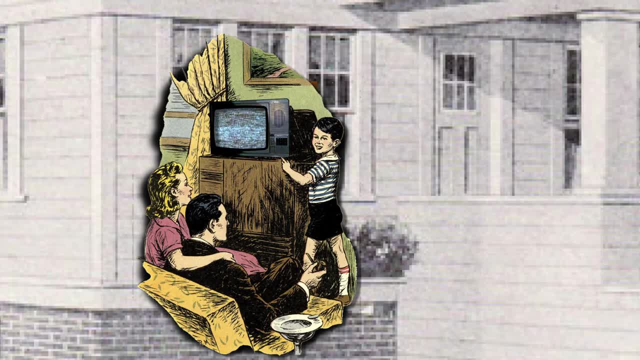 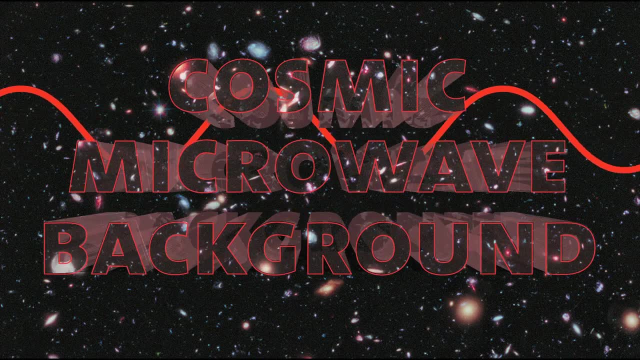 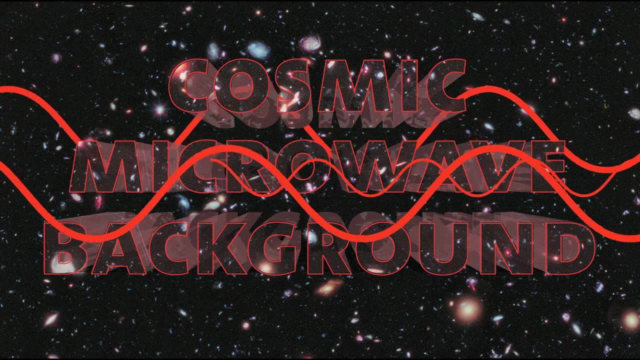 A few percent of the noise that you get when you tune to an empty channel was from the early universe. Those radio waves are what we call the cosmic microwave background, So the background of microwaves that pervades the universe because they were emitted during the early expansion of the universe. 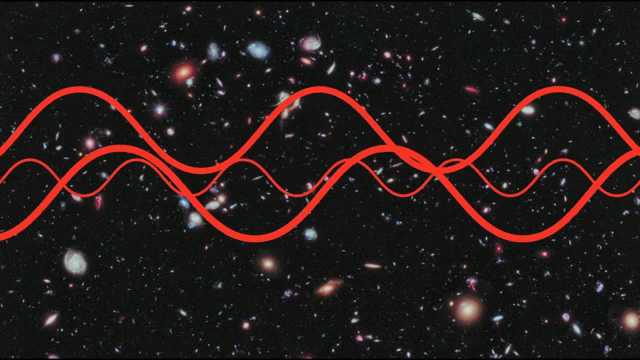 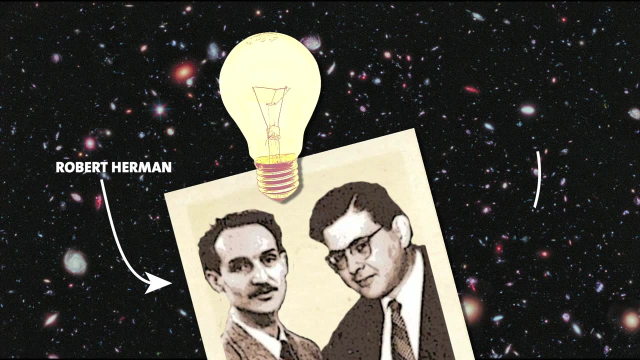 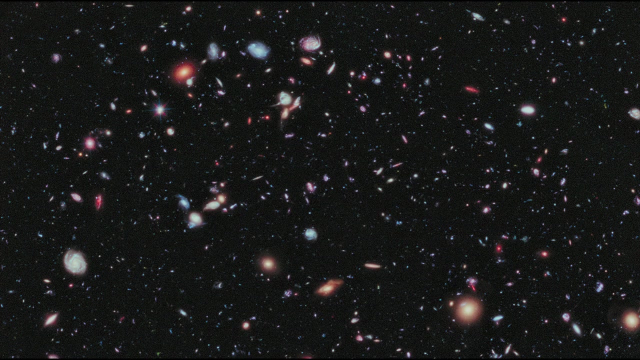 and have been traveling and getting stretched out ever since. The idea that there ought to be background radiation was actually first understood in the 1940s with the idea that there must be a hot, dense beginning to the universe. But sad to say, that prediction was more or less ignored for many years. 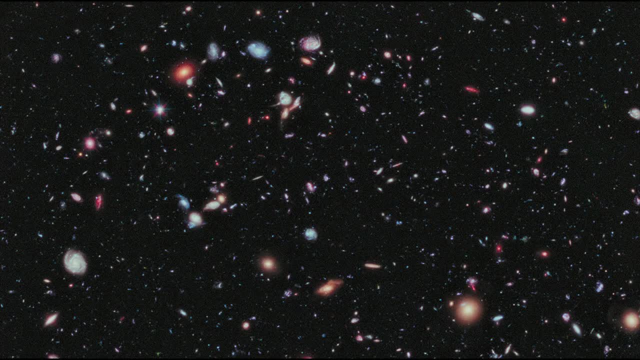 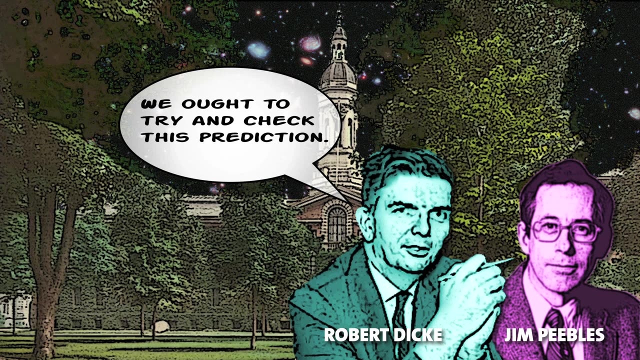 And it wasn't until the 60s that Peebles and Dickey at Princeton University, said we ought to try and check this prediction and set out to do so. Well, by the 60s, technology had advanced, the space race had started. 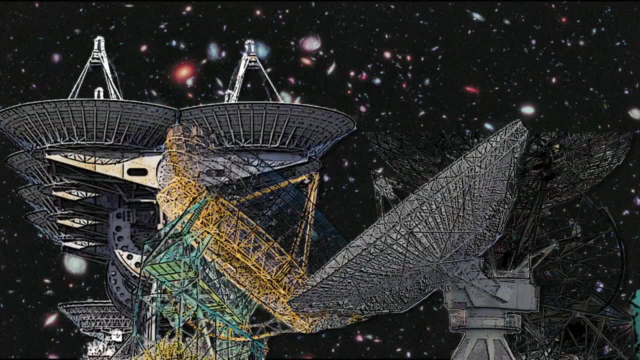 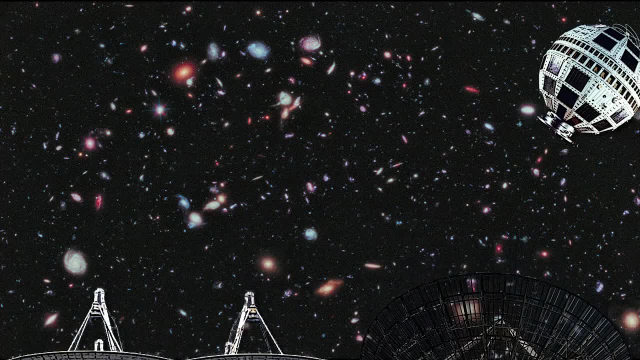 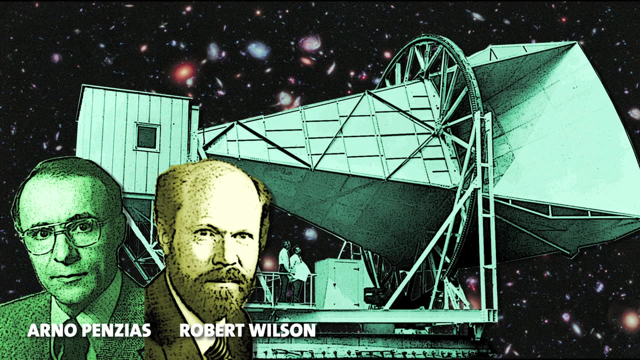 people were building microwave antennae, not to look for some crazy idea of some physicist sitting in a lab somewhere, but to follow communication satellites, And a couple of electrical engineers by the name of Penzias and Wilson got a hold of one of these antennae that had been used to follow the echo communication satellite. 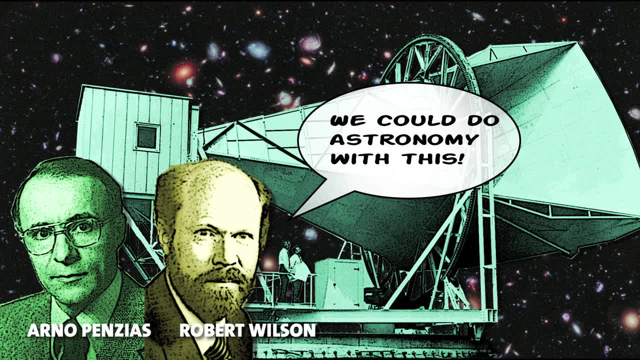 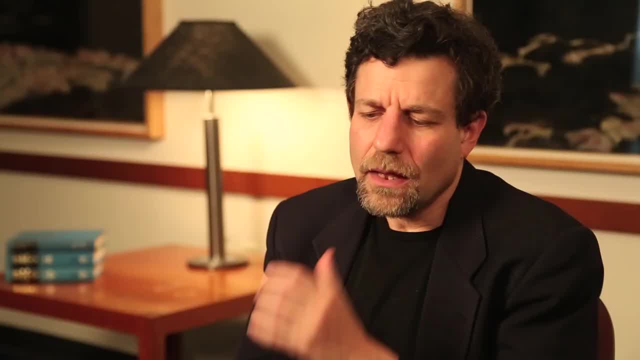 and thought to themselves: we could do astronomy with this, And so they started using it to try to detect emission from gas in the Milky Way galaxy. Now they were rather good engineers, And so the first thing they did was point their antennae at empty channels. 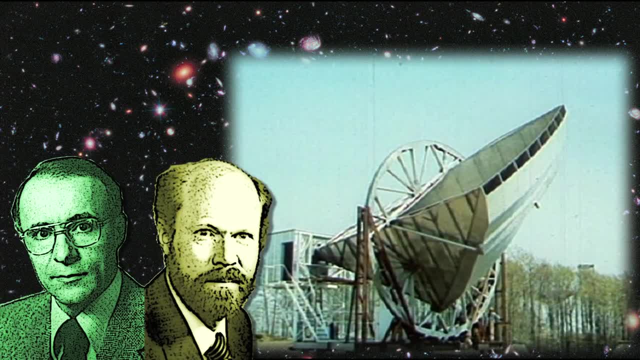 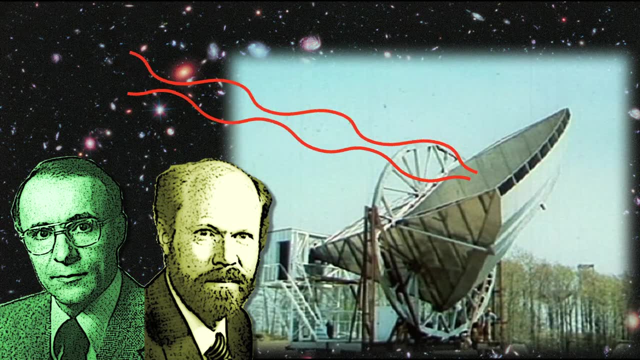 a patch of sky so they would be able to measure its noise level. And darn it all, there's something wrong with the system. They had too much noise. That is, their antennae was detecting a signal which they interpreted as noise.